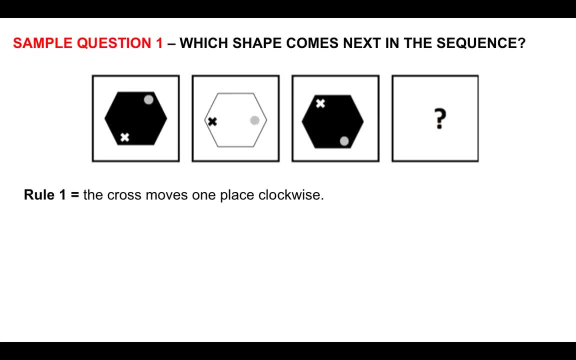 patterns straight away. There's a lot of rules which are applied and you have to work out what they are to get to the answer. So if you notice rule one, the cross moves one place clockwise. So that's the cross there. Now, on the next shape, it moves one place clockwise, which. 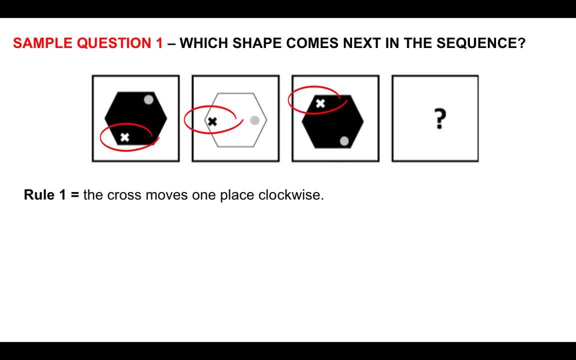 is obviously to the right, as the way a clock would go, and it moves there And it also alternates from white to black to white as it moves round. So we are looking for in the question mark one the next shape for the cross to be there. Then there's rule two. 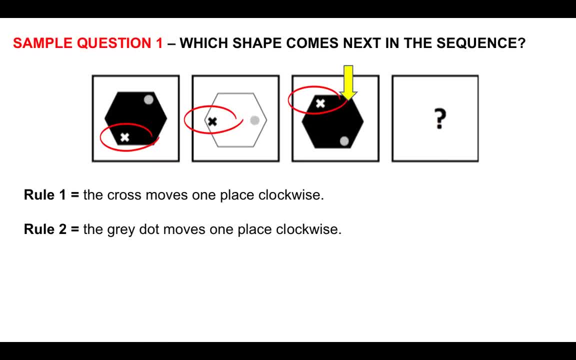 Now you'll notice that the gray dot moves one place clockwise as well. So that moves one place clockwise. So you've got the gray dot there. It stays consistent in the fact it is gray, but it moves one there, then it moves there. So in the next shape it needs. 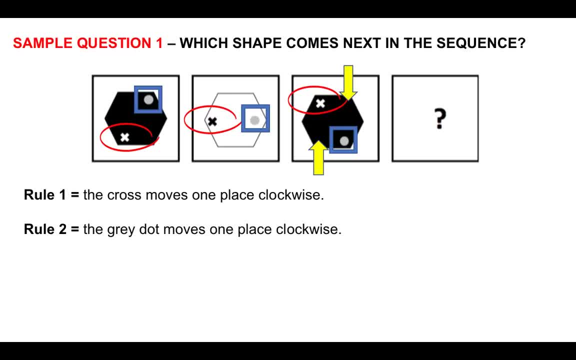 to be there. So in our head we can work out straight away: that's where they need to be. And, trust me, once you practice loads of these- and I'm going to give you some free sample test questions in a little while- then it becomes easy to answer these questions. There's also one other rule, which is rule two, Rule three, Rule four, Rule five, Rule six, Rule seven. Rule eight, Rule nine, Rule ten. Rule eleven: Rule twelve: Rule twelve. Rule thirteen. Rule sixteen: Rule eighteen: Rule sixteen: 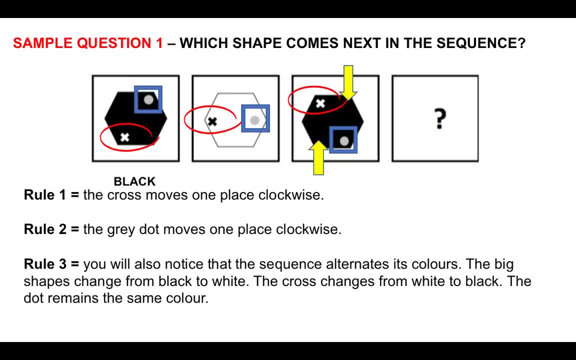 Rule nineteen, Rule nineteen, Rule twenty, Rule twenty, Rule twenty-one, Rule twenty-one. And we've got the same rule, but this time it's really obvious and that is the fact that, you'll notice, the sequence alternates from black to white to black, So we are looking. 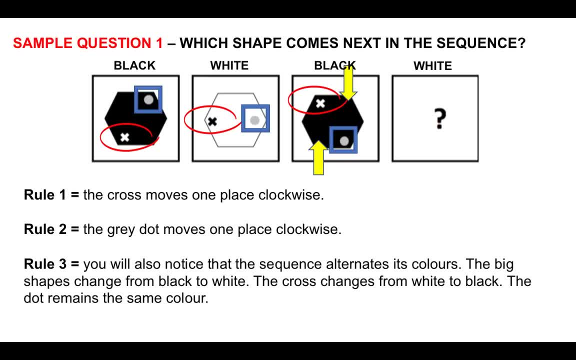 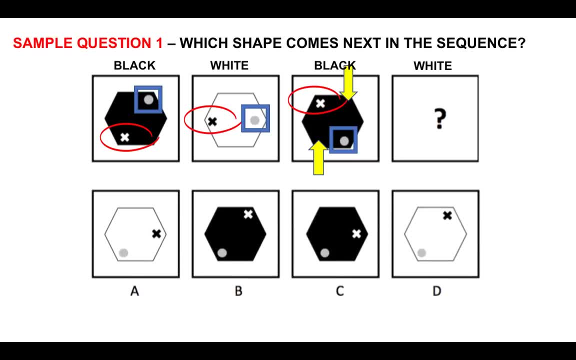 for something that is white. And this is a great tip- is when you're answering these questions and you automatically straightaway work out a sequence. if we put up the options there, you can eliminate straightaway the black shape. So you are just left with A. 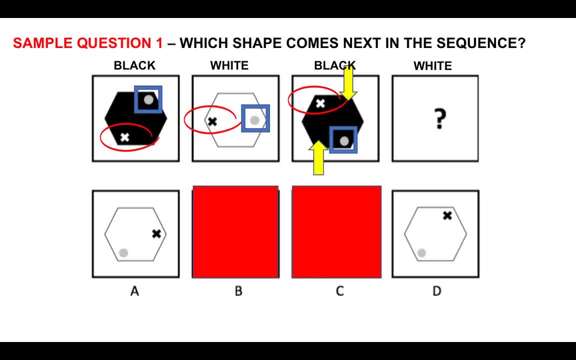 or D And, in a worst case scenario, if you were running out of time and you wanted to do some guessing, which is not always advised, But you know, so long as you don't lose marks for guessing, then you could just go well. 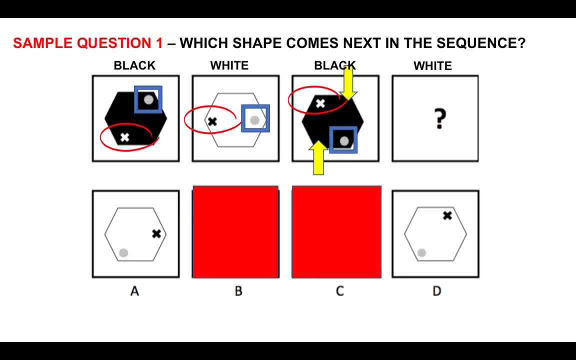 it's going to be a white one. I'll choose between A or D And you've got a 50-50 chance of success. So we can see there that the correct answer is D. So D is the answer to sample question one. 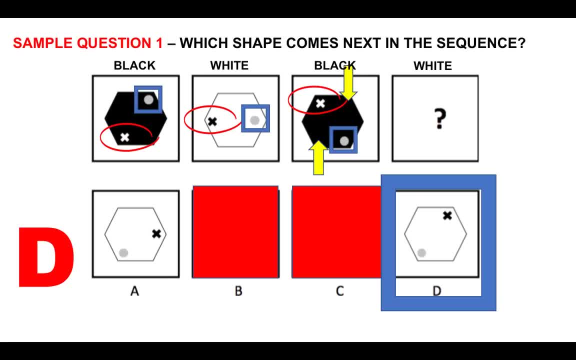 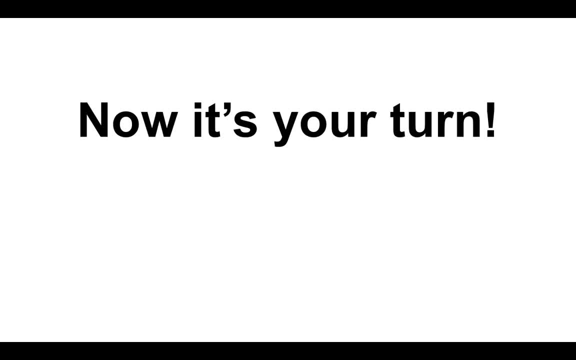 And, like I say, you'll become so good at these once you practice loads of these questions and understand and apply the list that I'm going to show you soon what to look out for. So now it's your turn. I've got question two. 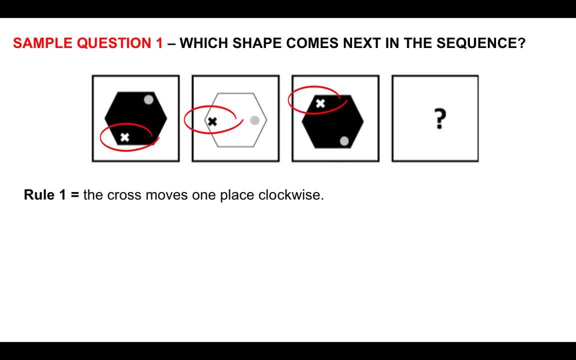 is obviously to the right, as the way a clock would go, and it moves there And it also alternates from white to black to white as it moves round. So we are looking for in the question mark one the next shape for the cross to be there. Then there's rule two. 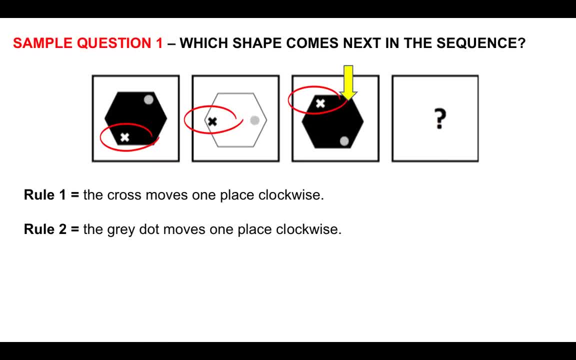 Now you'll notice that the gray dot moves one place clockwise as well. So that moves one place clockwise. So you've got the gray dot there. It stays consistent in the fact it is gray, but it moves one there, then it moves there. So in the next shape it needs. 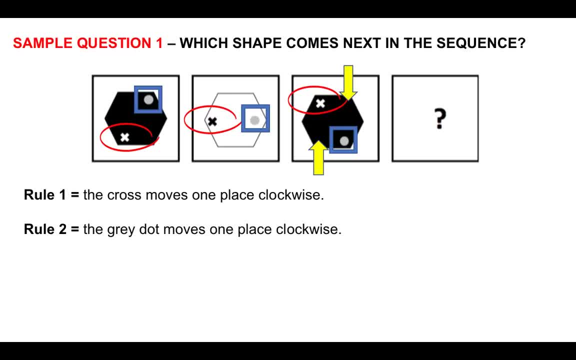 to be there. So in our head we can work out straight away: that's where they need to be. And, trust me, once you practice loads of these- and I'm going to give you some free sample test questions in a little while- then it becomes easy to answer these questions. 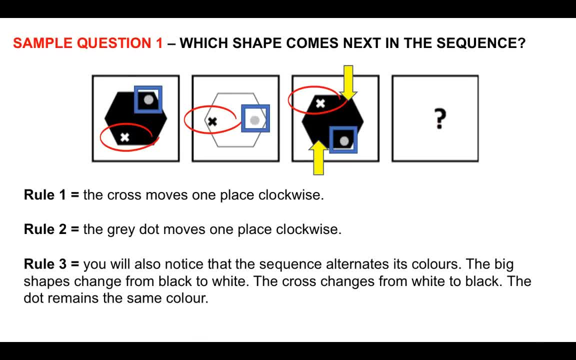 There's also one other rule, which is rule two, Rule three, Rule four, Rule five, Rule six, Rule seven, Rule eight, Rule nine, Rule ten, Rule twelve, And this is really obvious, and that is the fact that you'll notice the sequence. 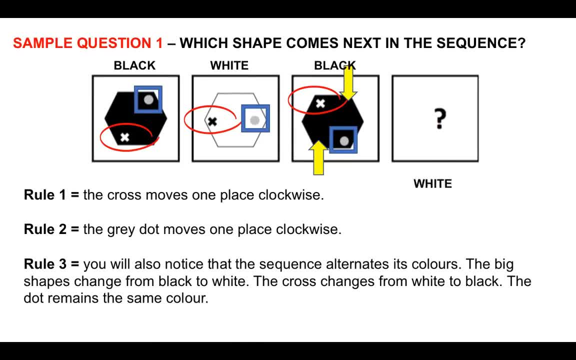 alternates from black to white to black, So we are looking for something that is white. And this is a great tip is when you're answering these questions and you automatically, straight away work out a sequence. if we put up the options there that you can eliminate straight. 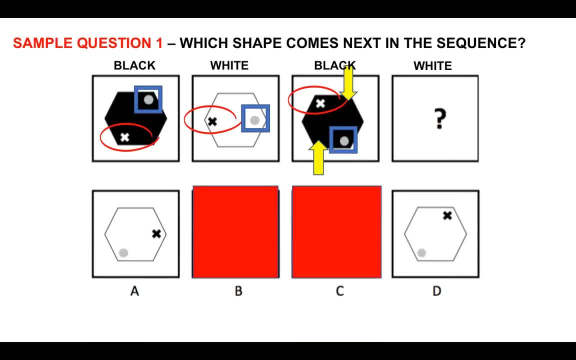 away the black shape, So you are just left with A or D And, in a worst case scenario, if you are running out of time and you wanted to do some guessing- which is not always advised, but as long as you don't lose marks for guessing, then you could just go. well, it's going to be a. 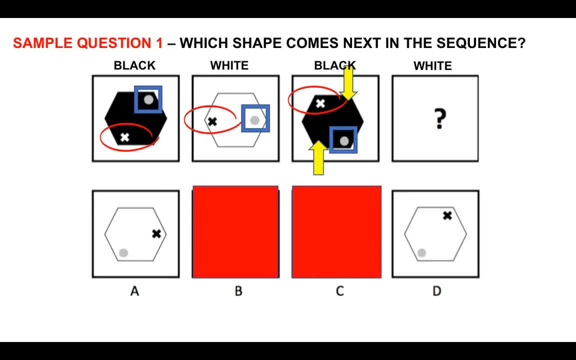 white one. I'll choose between A or D and you've got a 50-50 chance of success. So we can see there that the correct answer is D. So D is the answer to sample question one And, like I say you'll. 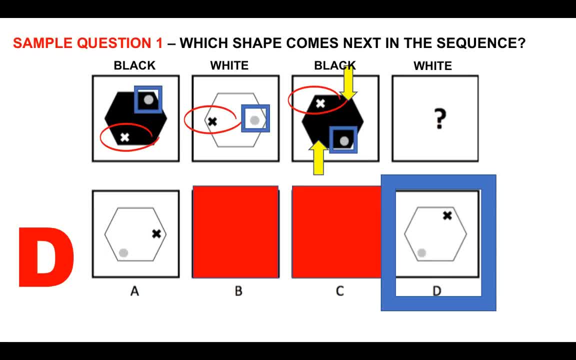 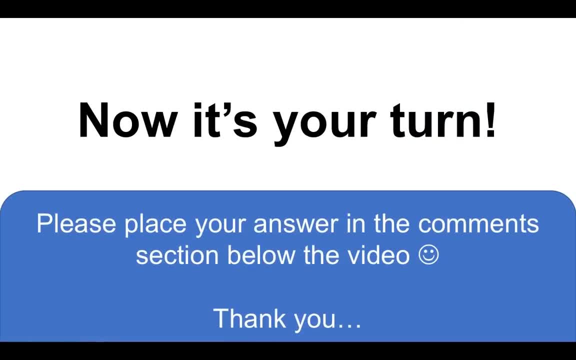 become so good at these once you practice loads of these questions and understand and apply the list that I'm going to show you soon what to look out for. So now it's your turn. I've got question two. Please place your answer in the comments section below the video and I'll come on each. 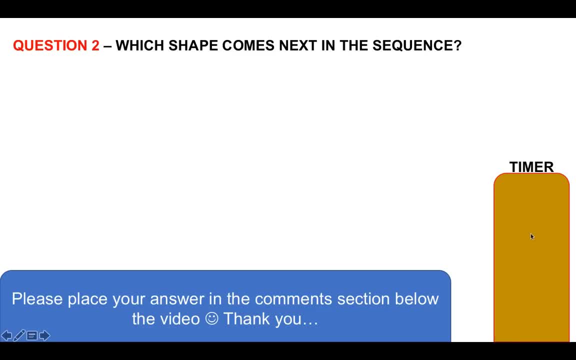 day and mark them. Question two: There's a timer there on the right-hand side, So I'm going to give you 15 seconds to answer this one. So which shape comes next in this sequence? Okay, So look out for the movement, the rotation of the star. Look at the lines as well to see whether there's any clues. 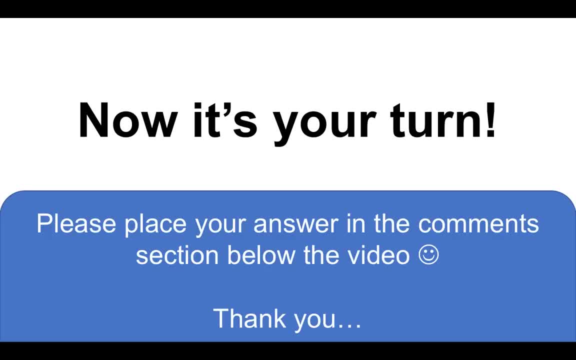 Uh, please place your answer in the comment section below the video and I'll come on each day and mark them. Question two: There's a timer there on the right hand side, So I'm going to give you 15 seconds to answer this one. 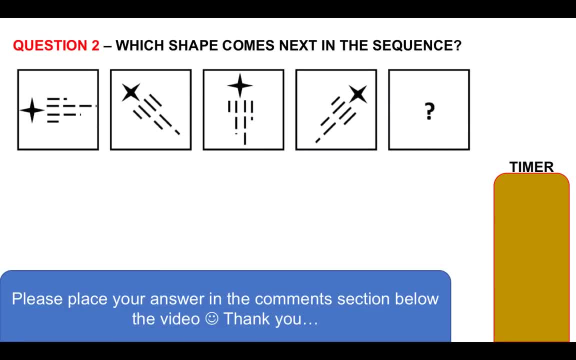 So which shape comes next in this sequence? Okay, So look out for the movement, the rotation of the star. Look at the lines as well to see whether there's any clues as to what you're looking out for Now. the options are A, B, C, D or E. 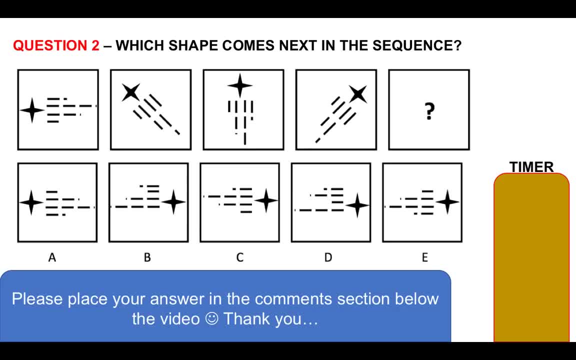 Now please put your answer in the comment section Below to question number two. I'll give you 15 seconds to answer. that. It looks easy, but don't forget to double check which is the right one, because there's a few options there which it could be. 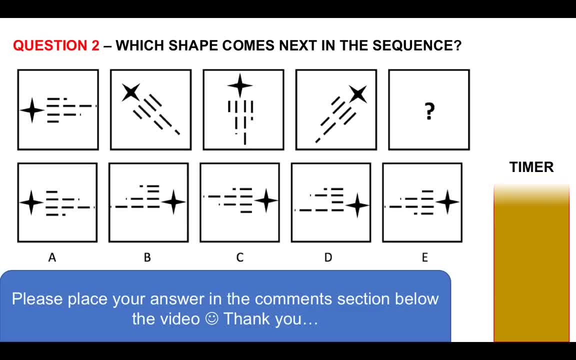 Off you go, guys. So not as straightforward as it seems. Like I say, if you need more time, just pause the video, but please put your answer to question two in the comments section below. Okay, Question number three. Which shape completes the sequence. 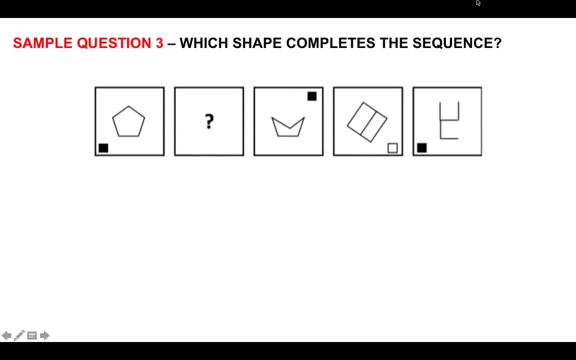 Now, this is a bit of a tricky one, because, if you notice, there, they're asking us to find out what goes there, What not comes next in the sequence, but what completes it, And this is another variation of an abstract reasoning test. 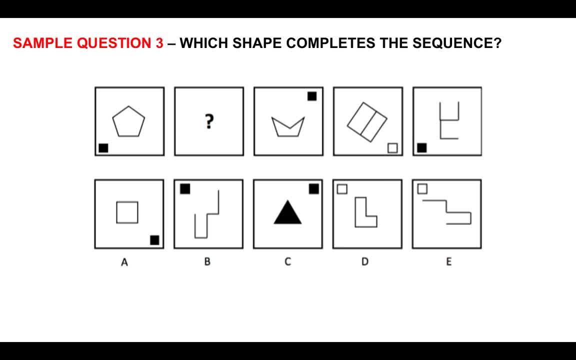 So these are the options there: A, B, C, D or E. So there's a couple of patterns there straight away that we can see. So you'll notice there that the black square again it's moving 90 degrees clockwise. 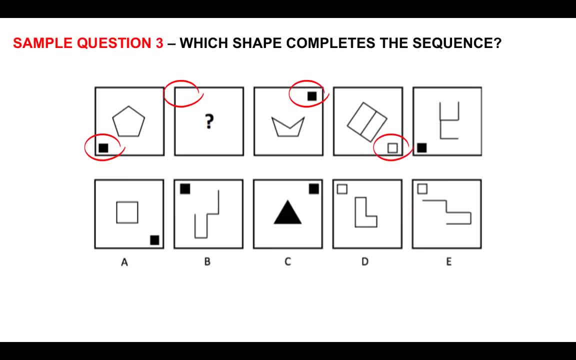 But you'll notice, there there's a white one and then there's a black one, So that tells me the one in there where the question mark is. it's got to be white, So automatically we could get rid of B and C if we wanted to straight away. 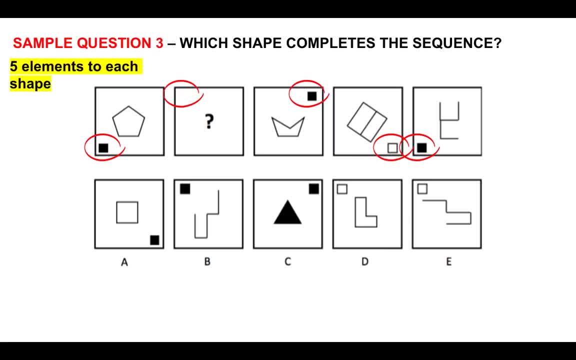 Now, you'll also now see, and this is where you need to do loads of practice, because I can tell, even though these shapes, there's no real rhyme or reason for these shapes, but they have all one thing in common and they have five elements or sides to them. 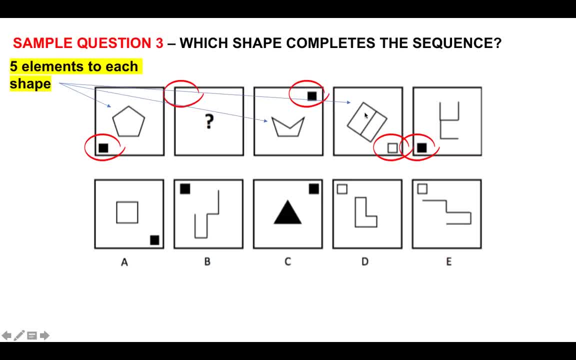 So that's got five sides there, That's got five, That's got five parts and that's got five parts. So automatically we can get rid of A, we can get rid of C, we can get rid of a, D. 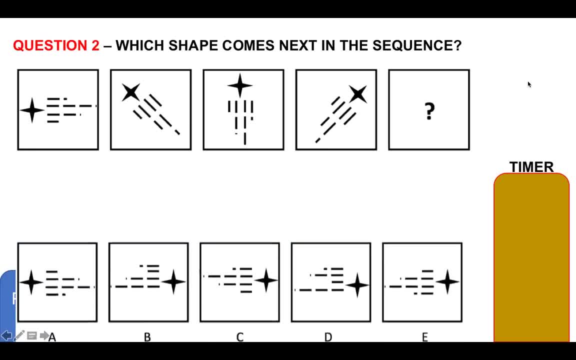 as to what you're looking out for Now. the options are A, B, C, D or E. Now please put your answer in the comments section below the video and I'll come on each day and mark them. Question two: 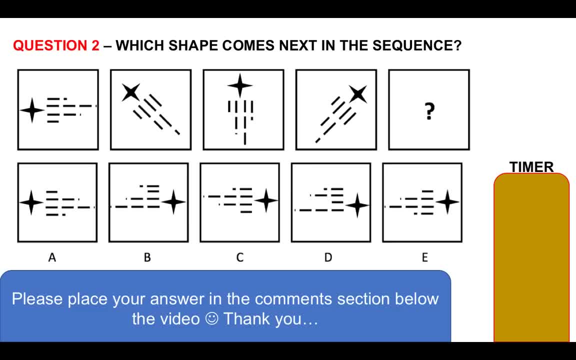 Please place your answer in the comments section below to question number two. I'll give you 15 seconds to answer that. It looks easy, but don't forget to double check which is the right one, because there's a few options there which it could be Off you go, guys. 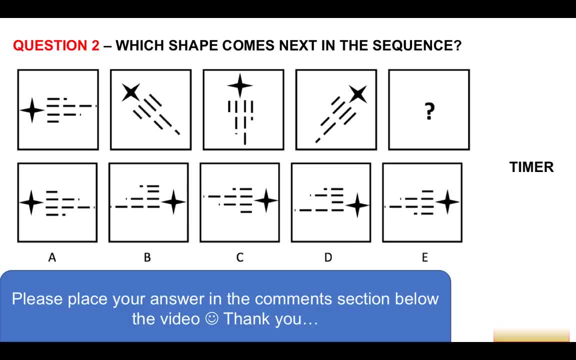 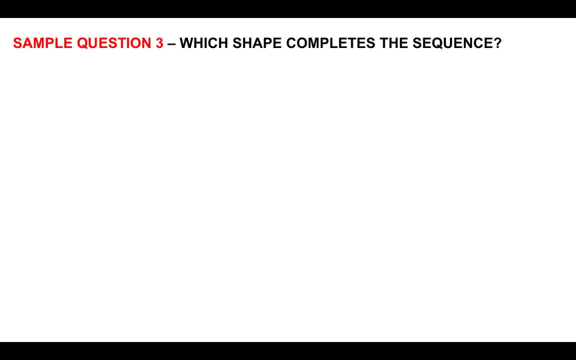 So not as straightforward as it seems. Like I say, if you need more time, just pause the video, but please put your answer to question two in the comments section below. Okay, Question number three, which shape, completes the sequence. Now, this is a bit of a tricky one. 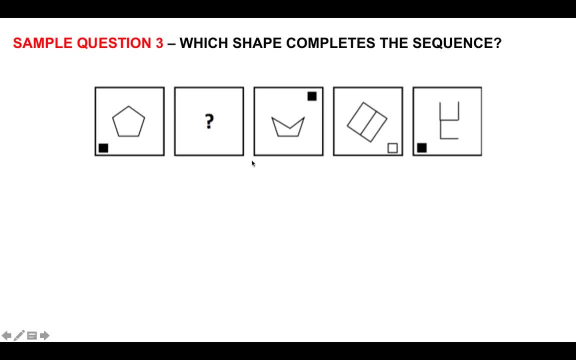 because, if you notice, there they're asking us to find out what goes there, what not comes next in the sequence, but what completes it. And this is another variation of an abstract reasoning test. So these are the options there: A, B, C, D or E. So there's a couple of patterns there, straight. 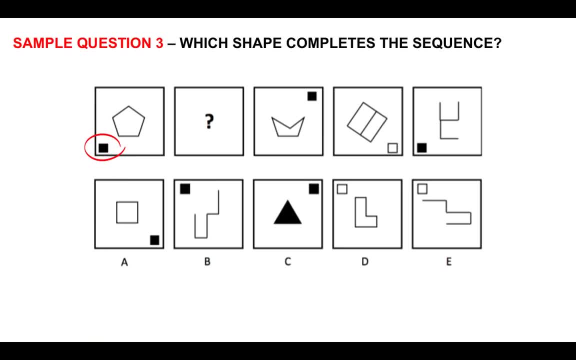 away that we can see. So you'll notice there that the black square, again it's moving 90 degrees clockwise. So it's moving 90 degrees clockwise. So it's moving 90 degrees clockwise. So it's moving 90 degrees clockwise around. But you'll notice there there's a white one and then there's a black. 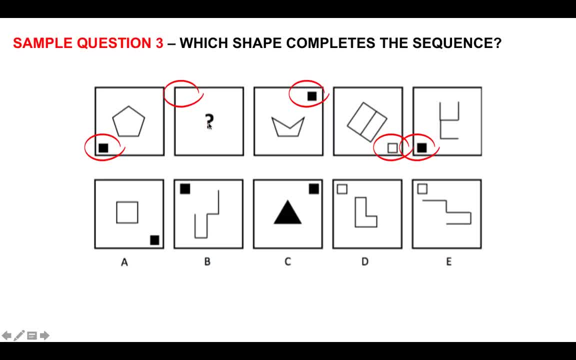 one. So that tells me the one in there where the question mark is. it's got to be white, So automatically we could get rid of B and C if we wanted to, straight away Now you'll also now see- and this is where you need to do loads of practice. 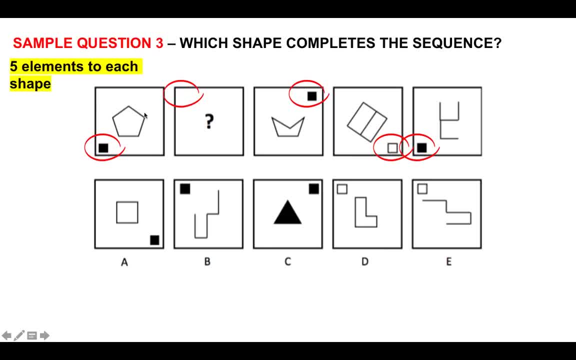 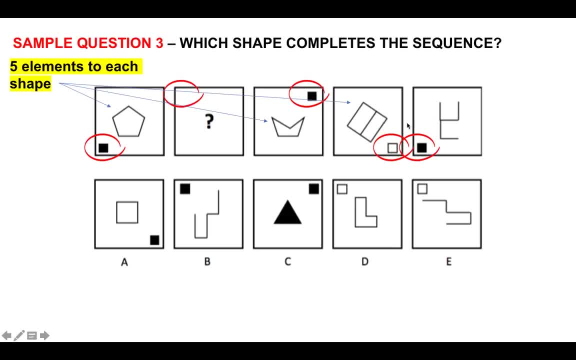 five elements or sides to them. So that's got five elements or sides to them. So that's got five elements there, That's got five, that's got five parts and that's got five parts. So automatically we can get rid of A, we can get rid of C, we can get rid of D, So it's either B or E. Well, 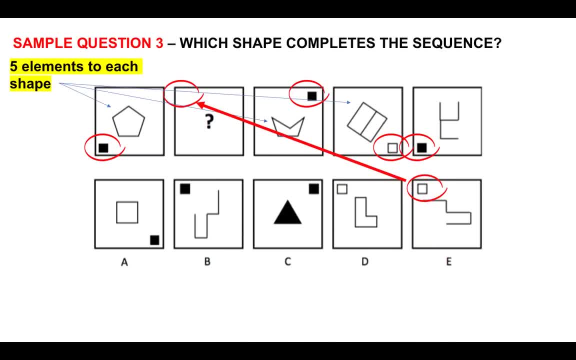 automatically. we know we need a white one and it needs to be placed there. So it's either D or E, and the correct answer that's the only one with five elements. So the answer is E. So there you're looking at rotating shapes, 90 degrees, either clockwise or anticlockwise, but also how many? 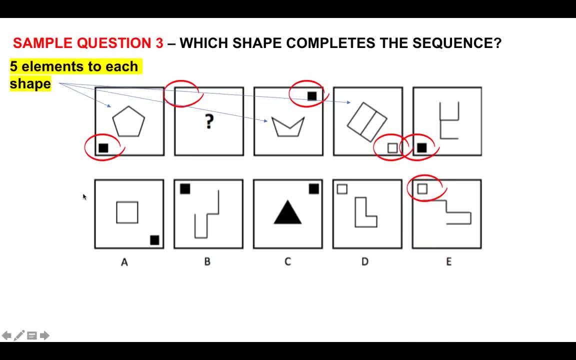 So it's either B or E? Well, automatically, we know we need a white one and it needs to be placed there. So it's either D or E and the correct answer that's the only one with five elements. So the answer is E. So there you're, looking at rotating shapes: 90 degrees, either clockwise. 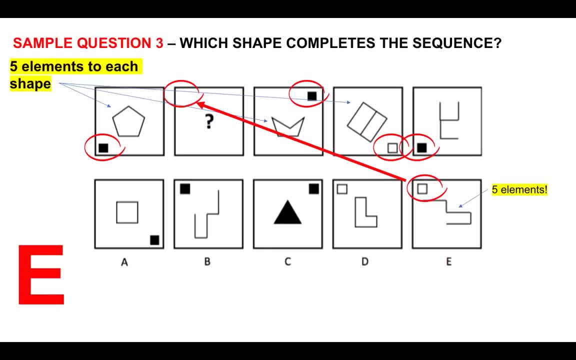 or anticlockwise, But also how many elements or sides there are. and a lot of people fail these tests because they're looking for consistency in shapes, and it's not about that. This is just simply. they've got five elements to them. 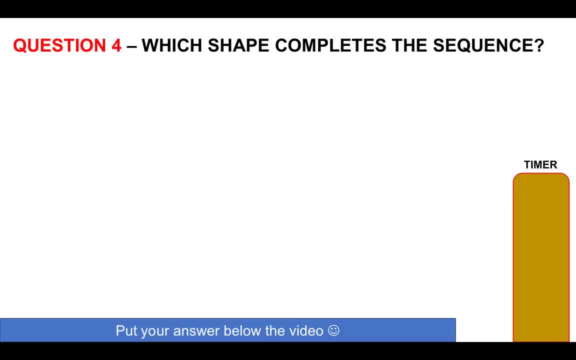 So you need to look out for that and, like I say, the more of these you do, the better. Okay, now it's your go. again, guys, I've got a question, for which shape completes the sequence? Okay, so look for patterns, look for variations. 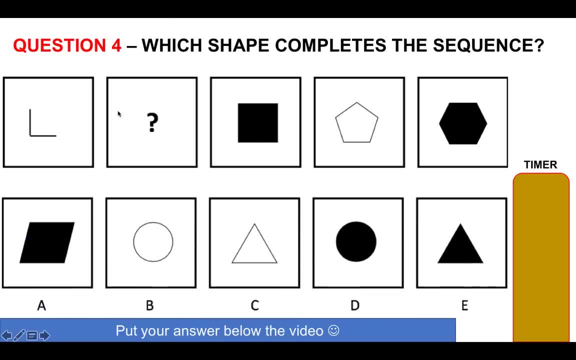 Which shape completes the sequence You're looking at? which one goes there with a question mark? There's the options A, B, C, D or E. I'll give you 15 seconds and, like I say, if you need more time, please. 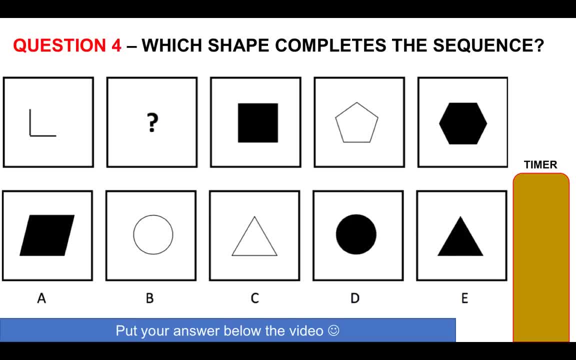 feel free to pause the video, but once you've done it, please put your answer to question four in the comments section below, and then we'll move on to the next one. Thank you, So it is actually alternating things there going on, alternating colors perhaps, and 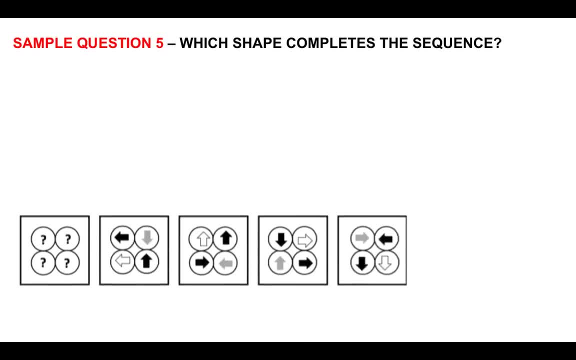 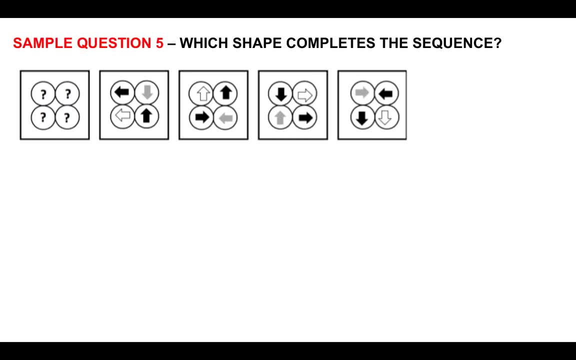 then different sides on shapes. Question number five: which shape completes the sequence? Now, this is a tougher one. okay, Now look out for this, because this can happen quite a lot in abstract reasoning tests. So which shape completes the sequence? So we need to find out which one starts it, not which one comes at the end, but which. 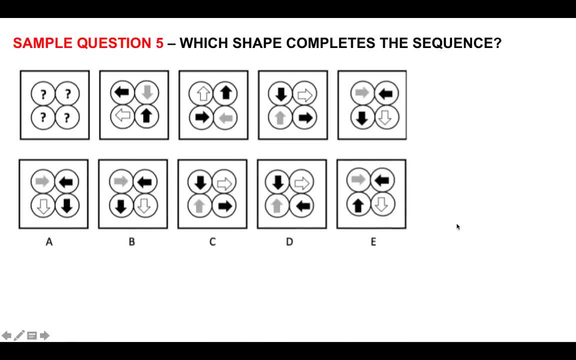 one here starts it. So these are the options. okay, And upon first inspection it looks really confusing, Trust me, it looks really confusing, but what we're going to do is we're going to try and start answering this question. We're going to start with this one here, the first one. 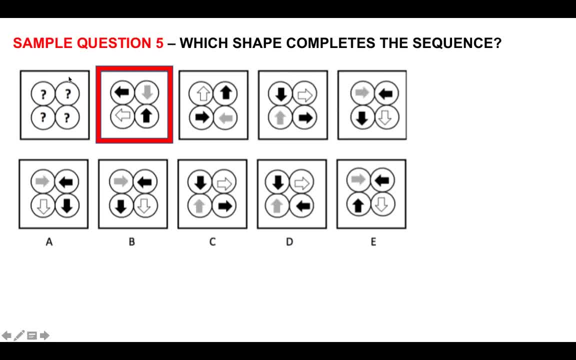 Now we're going to find out the sequence of what's going on that way, and then we can work backwards to the first one. okay, So let's just pick out that first shape and drop it there in our head. So we're looking at that now. 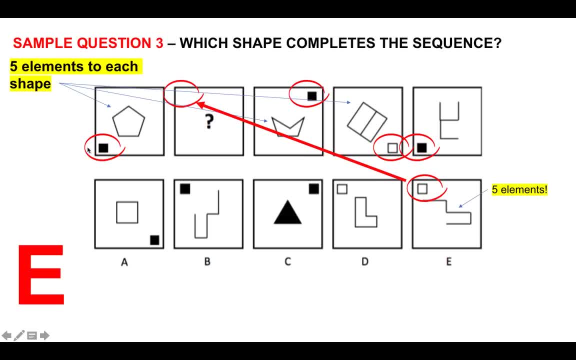 elements or sides there are, And a lot of people fail these tests because they're looking for consistency in shapes, And it's not about that. This is just simply they've got five elements to them, So you need to look out for that And, like I say, the more of these you do, the better. 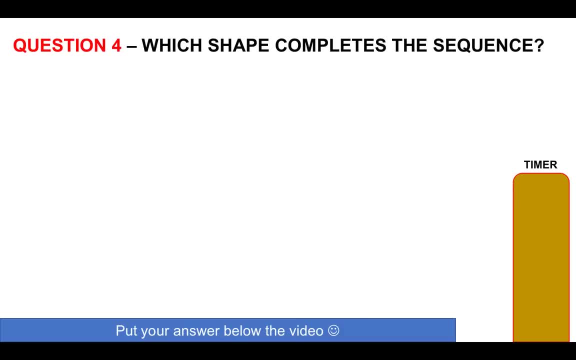 Okay, Now it's your go again. guys, I've got a question for which shape completes the sequence? Okay, So look for patterns, look for variations. which shape completes the sequence? You're looking at which one goes there with a question mark. There's the options A, B, C, D or E. 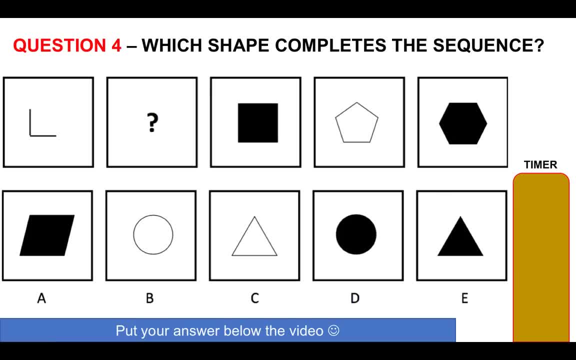 I'll give you 15 seconds And, like I say, if you need more time, please feel free to pause the video. But once you've done it, please put your answer to question four in the comment section below and then we'll move on to the next one. Thank you, So it is actually alternating things. 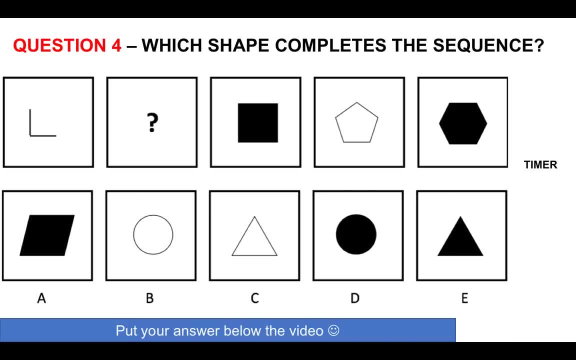 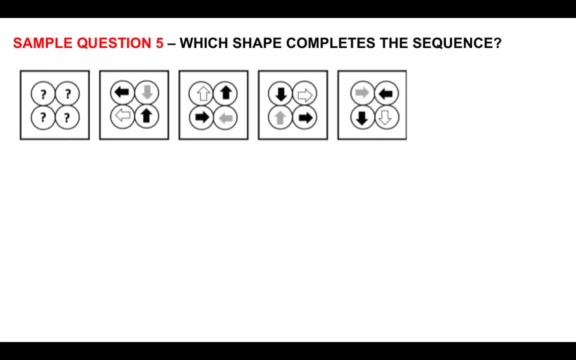 there going on alternating colors perhaps, and then different sides. on shapes. Question number five: which shape completes the sequence? Now, this is a tougher one. Okay, Now look out for this, because this can happen quite a lot in abstract reasoning tests. So, which shape completes the sequence? So we need to find out. 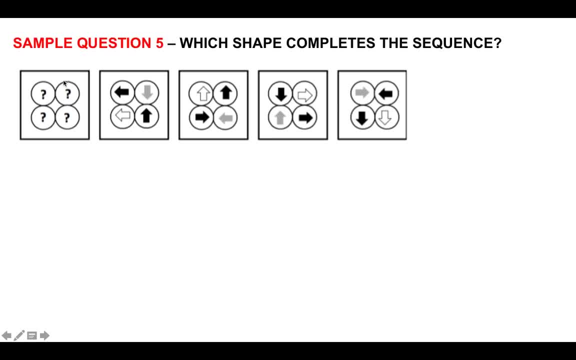 which one starts it, not which one comes at the end, but which one here starts it. So these are the options, Okay, And upon first inspection it looks really confusing. Trust me, it looks really confusing, But what we're going to do is we're going to try and start answering this question. 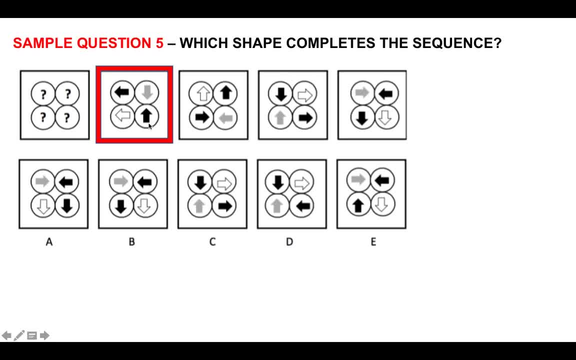 with this one here, the first one Now. we're going to try and start answering this question. with this one here, the first one Now. we're going to find out the sequence of what's going on that way, and then we can work backwards to the first one. Okay, So let's just pick. 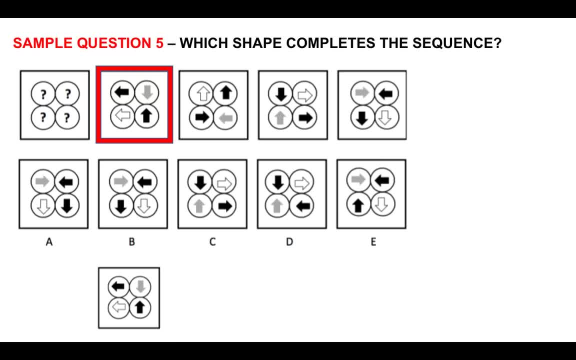 out that first shape and drop it there in our head. So we're looking at that now. Now, if you look at this- and this again is once you practice this kind of thing- you're looking for rotations. What is actually happening here? The entire shape is rotating 90 degrees. 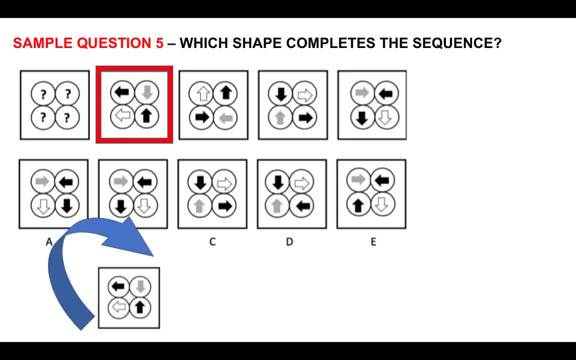 clockwise, not just individual shapes in the circles, but the whole one is just rotating 90 degrees. So if we turn this one here, the first one, 90 degrees to the right, it looks like that, which is exactly that one. Then if we move that one, 90 degrees again, we get 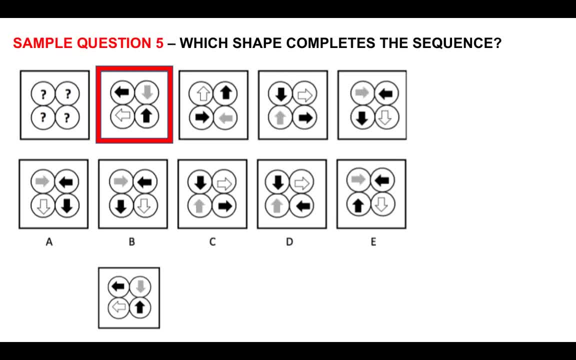 Now, if you look at this- and this again is, once you practice this kind of thing- you're looking for rotations. What is actually happening here? The entire shape is rotating 90 degrees clockwise, not just individual shapes in the circles. 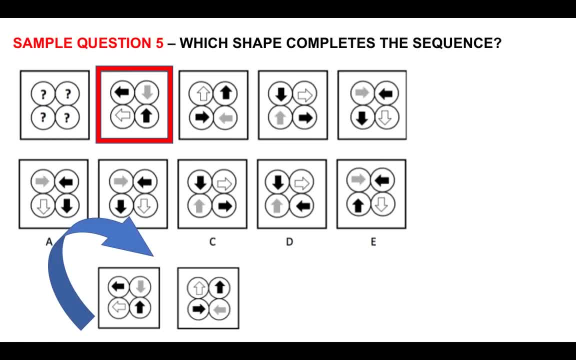 but the whole one is just rotating 90 degrees clockwise. Okay, So 90 degrees. So if we turn this one here, the first one, 90 degrees to the right, it looks like that, which is exactly that one. Then if we move that one, 90 degrees again, we get that one which is the exact same shape. 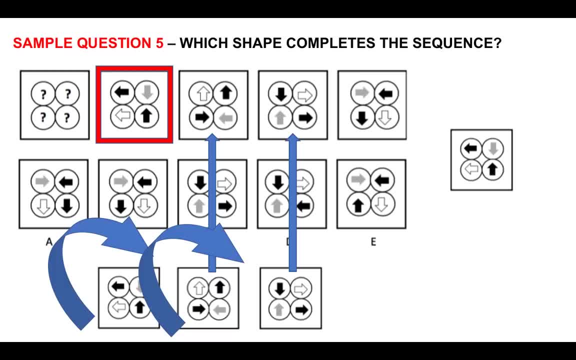 and so on and so forth. So to get the answer, let's take the first one, which is there again, and let's rotate it not 90 degrees clockwise but 90 degrees anti-clockwise, because we have to go the 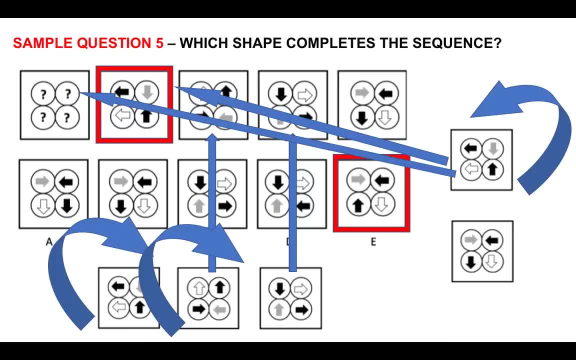 other way, because it's going to the left and not to the right. therefore, the correct answer is that It's E. Now, obviously, upon first inspection it looks really tricky and most people won't be able to answer that, but if you know what to look for in these kind of questions, it. 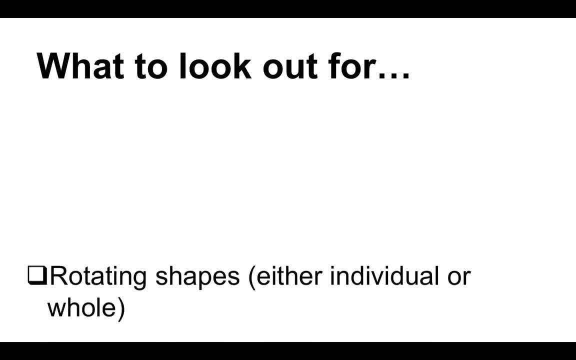 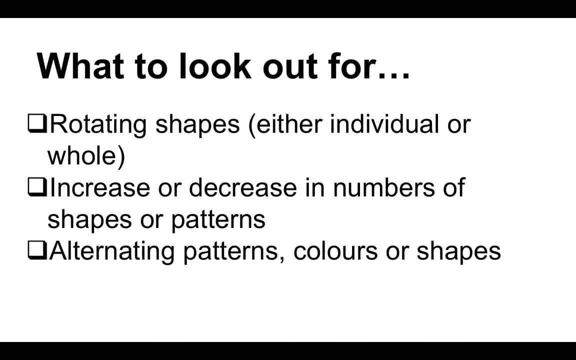 becomes relatively straightforward, and this is what to look out for. So take a note of these Rotating shapes, either individual shapes or as a whole. Now, in that last question, it was the entire shape that was rotated. Increases or decreases in the numbers of shapes or patterns, and also alternating patterns. 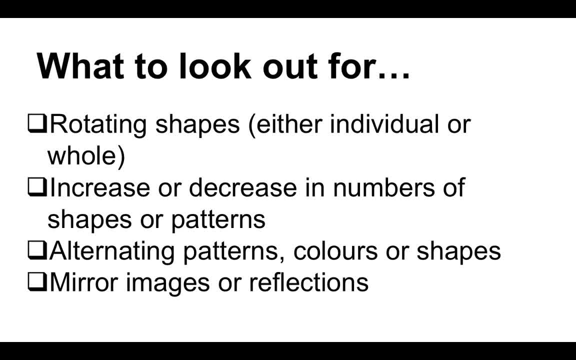 colors or shapes, And also mirror images or reflections. so where the patterns alternate, the colors change from black to white or whatever it is. But those are the four things, the key things to look out for. So now it's your turn again. 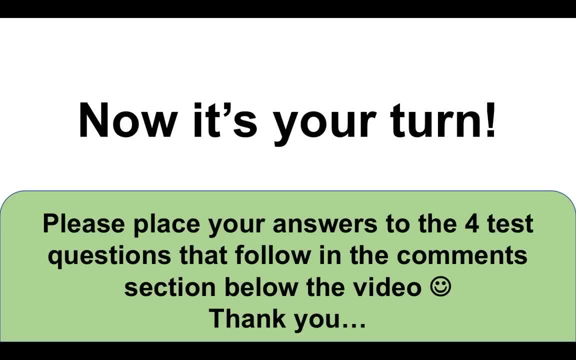 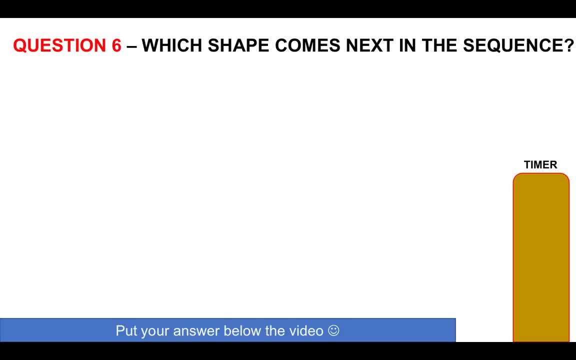 I'm going to give you four test questions to have a go at, of varying degrees. Again, please put your answer in the comments section below and once we've done these, I'm going to give you some more free test questions to have a go at. 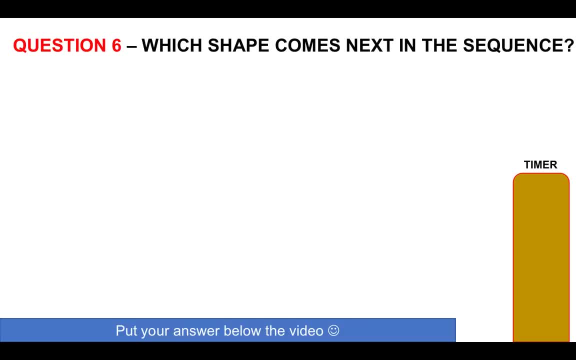 Like I say, don't forget. if you're liking the video, please give it a thumbs up. I really would appreciate that. I love making these videos for you guys. Questions to answer? Let me know in the comments. I'll be happy to answer them. 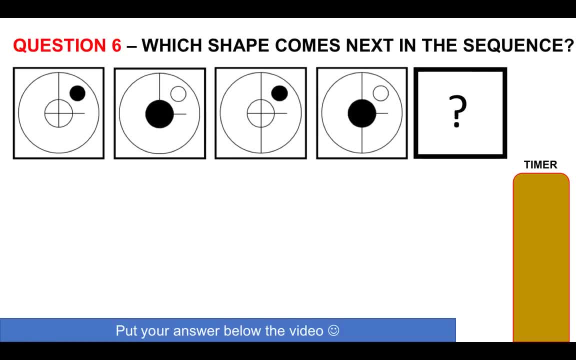 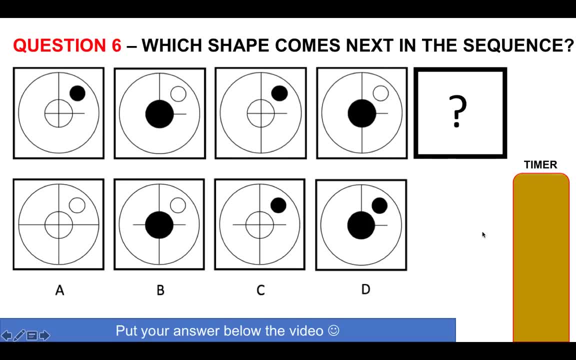 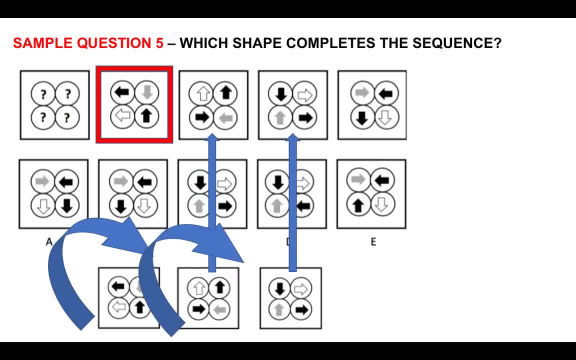 that one which is the exact same shape, and so on and so forth. So to get the answer, let's take the first one which is there again, and let's rotate it not 90 degrees clockwise, but 90 degrees anticlockwise, because we have to go the other. 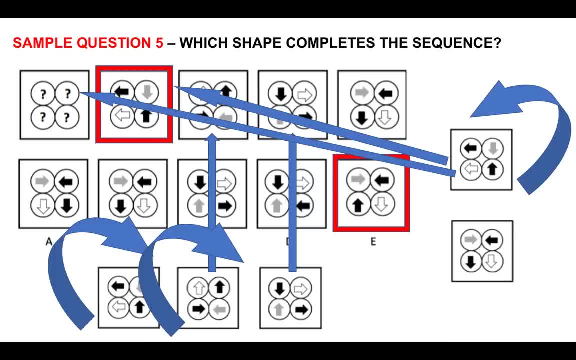 way, because it's going to the left and not to the right. Therefore, the correct answer is that which is E. Now, obviously, upon first inspection it looks really tricky and most people won't be able to answer that, but if you know what to look for in these kind of 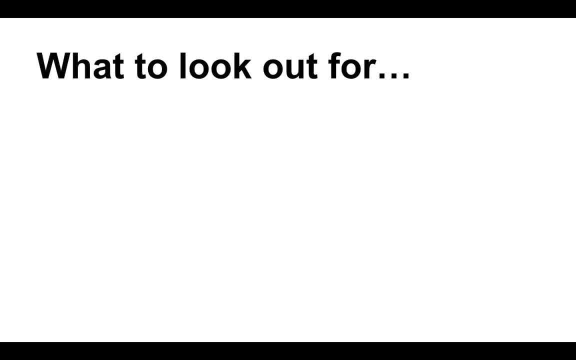 questions, it becomes relatively straightforward and this is what to look out for. so take a note of these Rotating shapes, either individual shapes or as a whole. Now, in that last question, it was the entire shape that was rotated. Increases or decreases in the numbers of shapes. 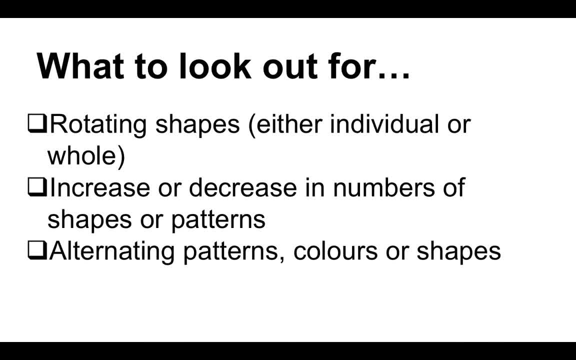 or patterns, and also alternating patterns, colors or shapes, and also mirror images or reflections. so where the patterns alternate, the colors change from black to white or whatever it is. but those are the four things, the key things to look out for. Now it's your. 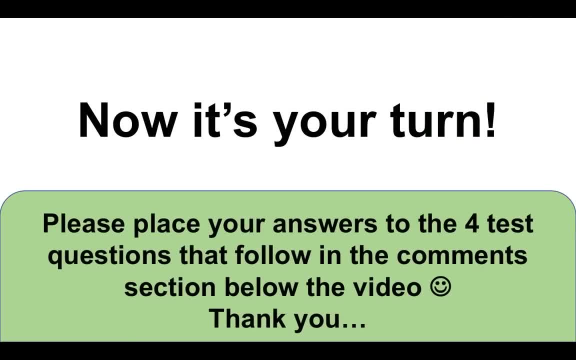 turn again. I'm going to give you four test questions to have a go at, of varying degrees. Again, please put your answer in the comments section below and once we've done these, I'm going to give you some more free test questions to have a go at. Like I say, don't. 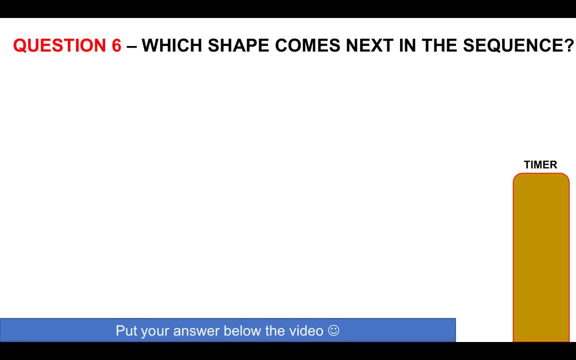 forget. if you like the video, subscribe to my YouTube channel and I'll see you in the next one. Please give it a thumbs up. I really would appreciate that. I love making these videos for you guys. Question six: which shape comes next in the sequence? So you're looking for. 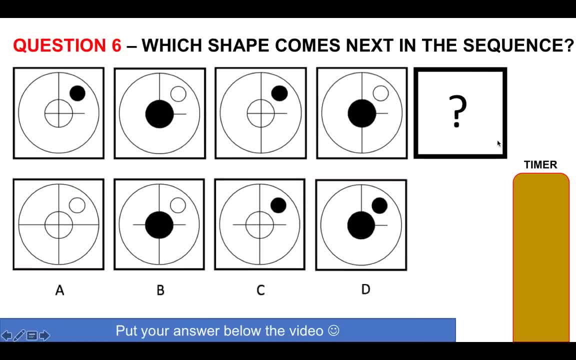 which one comes here. These are your options: A, B, C or D. I'm going to give you 15 seconds Off. you go, guys. Thank you. So don't forget what you've learned. Alternating colors increases. 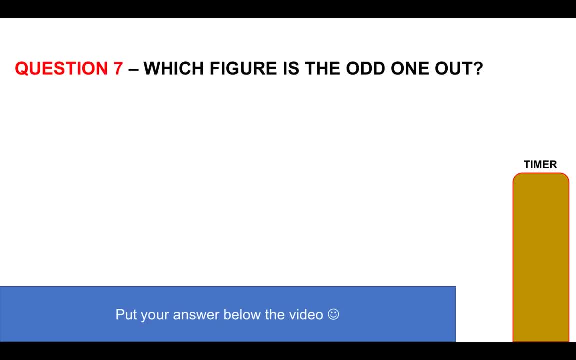 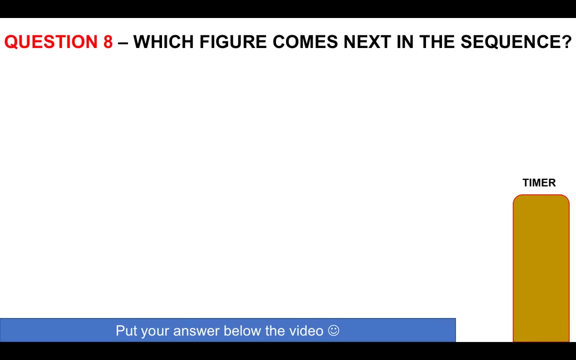 or decreases. decreases in shapes or movement of shapes. Question seven: Which figure is the odd one out, A, B, C or D? Please put your answer in the comments section below and also state why. Why is it which one you've chosen? Looks easy, but it's not Okay. Question number: 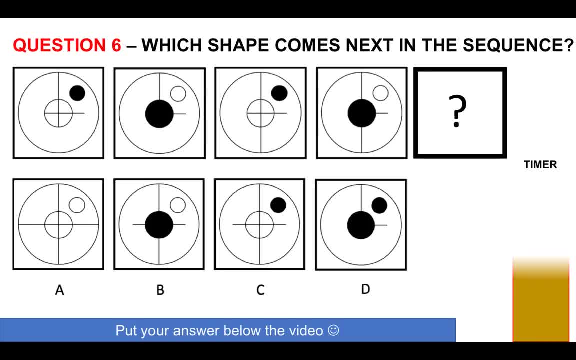 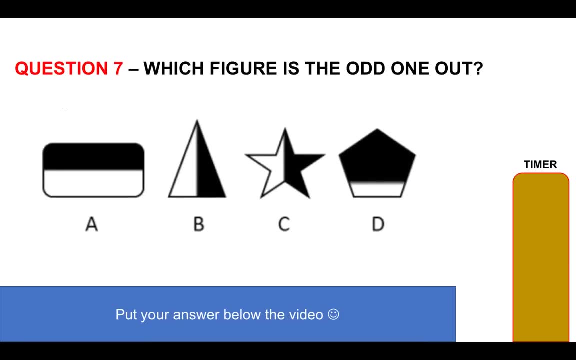 Thank you, So don't forget what you've learned. alternating colors, increases or decreases in shapes or movement of shapes. Question seven: Which figure is the odd one out, A, B, C or D? Please put your answer in the comments section below and also state why. 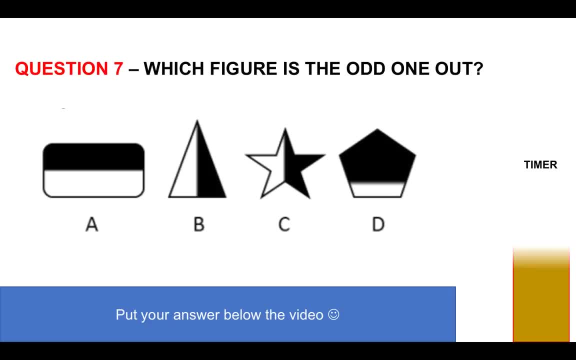 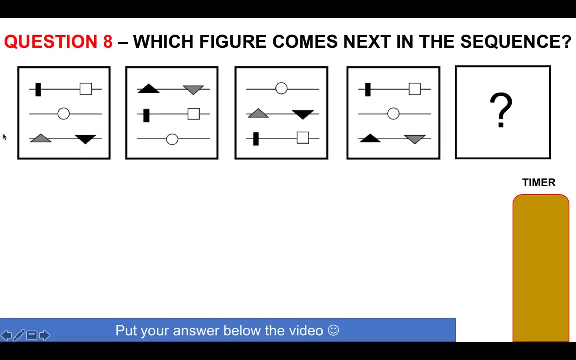 Why is it? which one you've chosen Looks easy, but it's not Okay. Question number eight: Which figure comes next in the sequence? So we're looking for one which goes there Now. remember what I said about movement of shapes and colors and patterns. 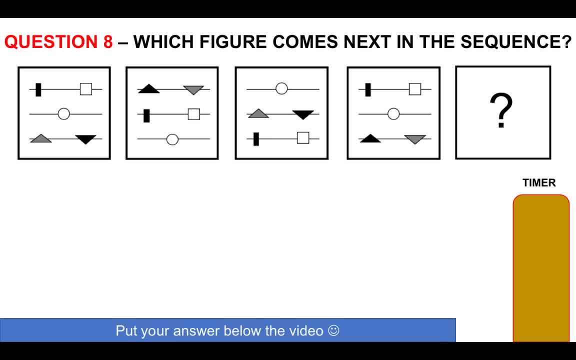 Have a look. Have a look which way the shapes are moving. Look for consistency in the shapes as well. Those are your answers: A, B, C or D. You might have to pause the video for this one, but I'll give you 15 seconds. 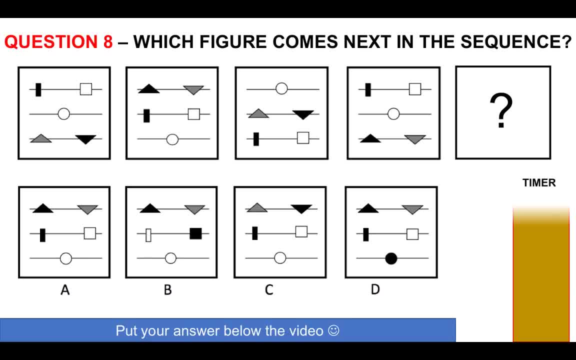 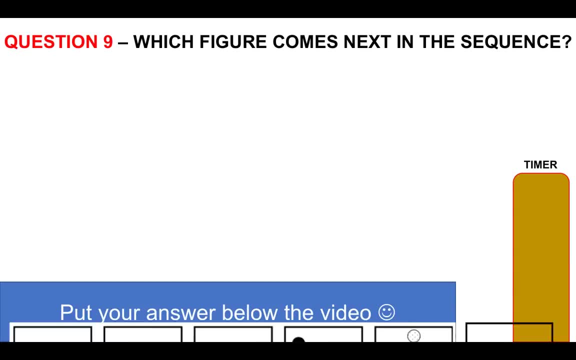 Off you go, guys. Thank you. If you're getting these right, then you're doing fantastic, Trust me. Question number nine: Which figure comes next in the sequence at the end? Again the odd one. Again, rotating of shapes, changes of patterns, etc. 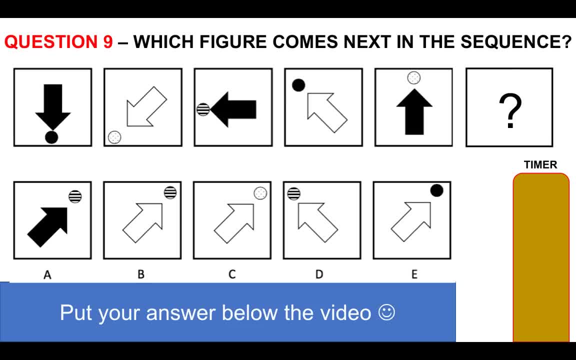 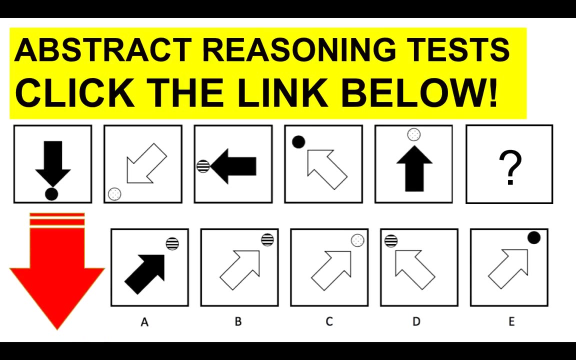 You've got A, B, C, D or E and you've got 15 seconds to answer this. Thank you, guys. So well done if you've reached or answered all of those questions and had a go at them. What I'd like to do now is click the link below the video and it will take you through. 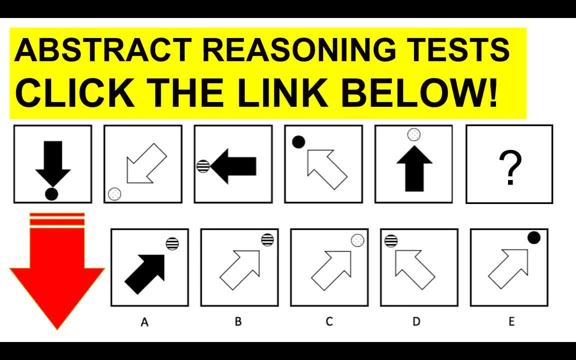 to my web page. You can get free access to more tests. Like I say, don't forget to put your answers to the questions and I'll comment and mark them every day. Hope you've enjoyed that video. Please, like I say, give it a thumbs up. 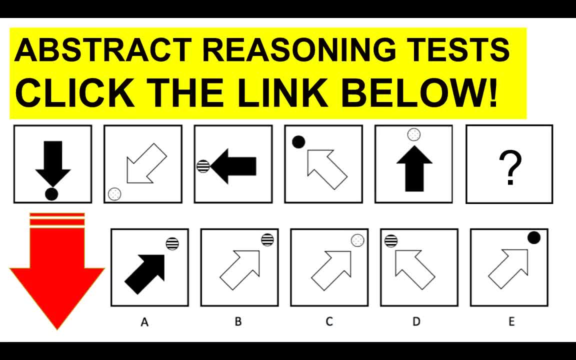 Really appreciate that. It'll motivate me to do more Love helping you guys. I'll also put a link below this video. If you want to download the slides to this presentation, you can get them on SlideShare. Just click the link below where it says Show More, and you can also connect with me on. 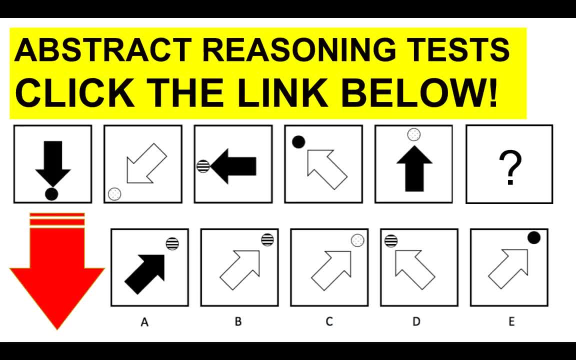 LinkedIn as well. Say hi. But thanks for watching and I wish you all the very best. guys And you're welcome. Have a wonderful pursuit to passing your Abstract Reasoning Test. Thank you,